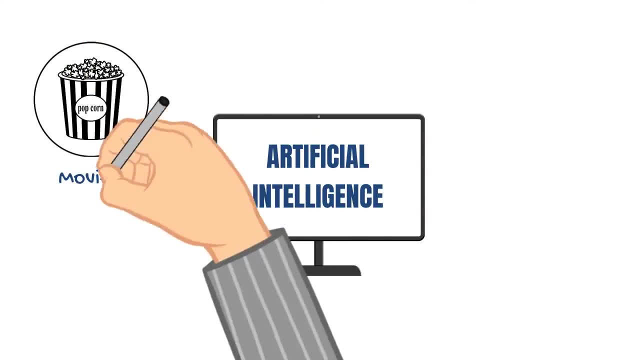 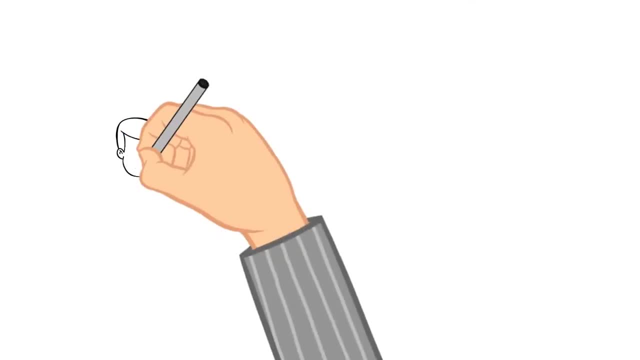 If you know about artificial intelligence mostly from movies and books, AI probably seems like this vague label for any machine that could think like a human. Fiction writers like to imagine a more generalized AI, one that answers any question we might have and do anything a human can do. 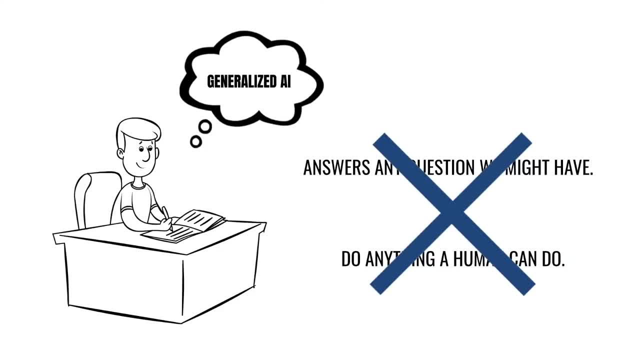 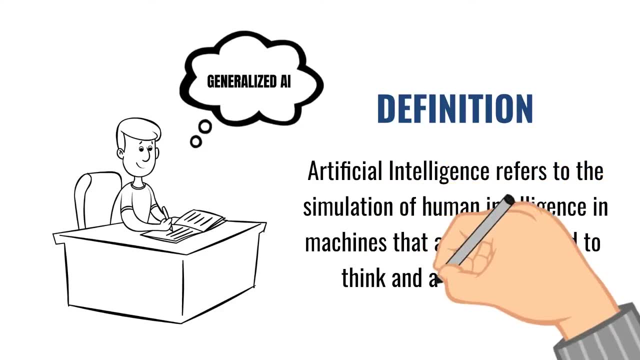 However, that's not the most realistic way to think about it. By definition, artificial intelligence refers to the simulation of human intelligence in machines that are programmed to think and act like humans. By using vast amounts of data and algorithms, AI technologies are able. 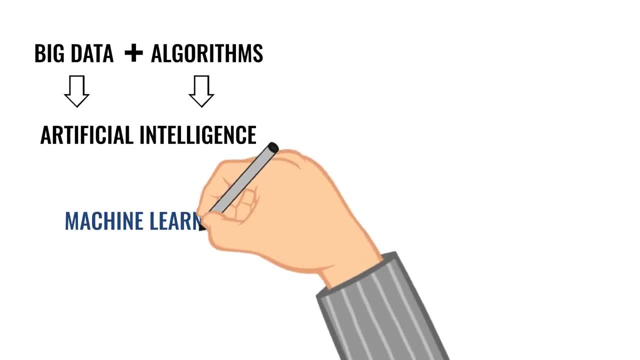 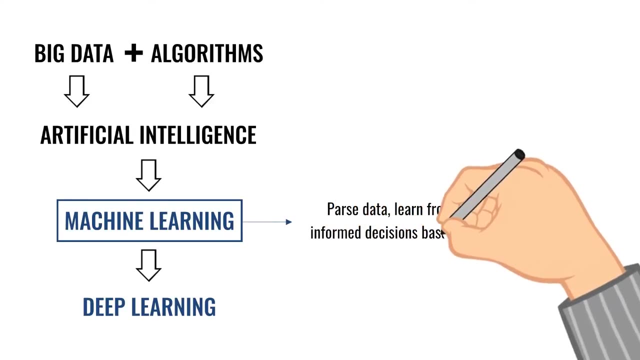 to achieve two important techniques: machine learning and deep learning. Both terms fall under the broad category of AI. However, machine learning is a subfield of artificial intelligence that uses algorithms to parse data, learn from that data and make informed decisions based on. 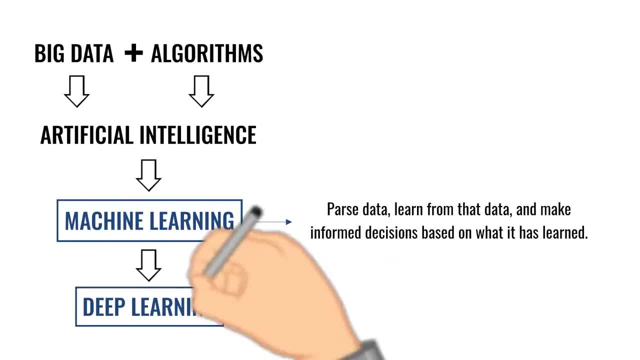 what it has learned. On the other hand, deep learning is a subfield of machine learning that uses algorithms to parse data, learn from that data and make informed decisions based on what it has learned. On the other hand, deep learning is a subfield of machine learning that 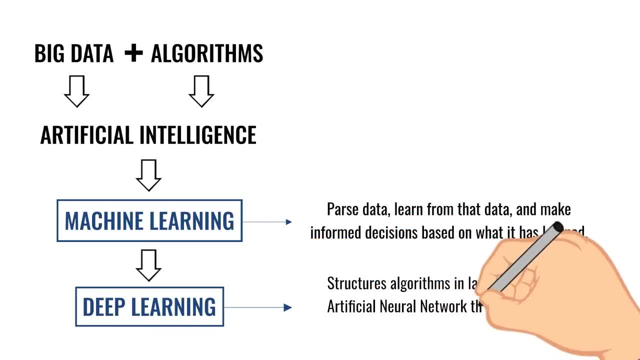 structures, algorithms in layers, to create an artificial neural network that can learn and make intelligent decisions on its own with even greater accuracy. The easiest example to differentiate both techniques is to think about Amazon Alexa, which recognized your voice commands without training, and the voice-to-type applications of a decade ago, which required 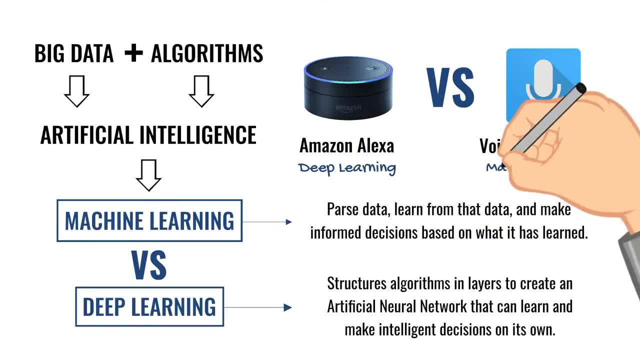 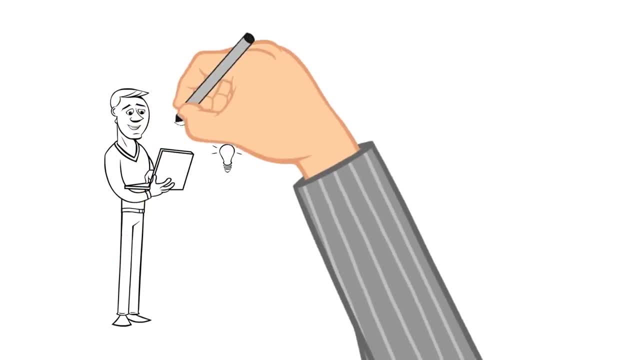 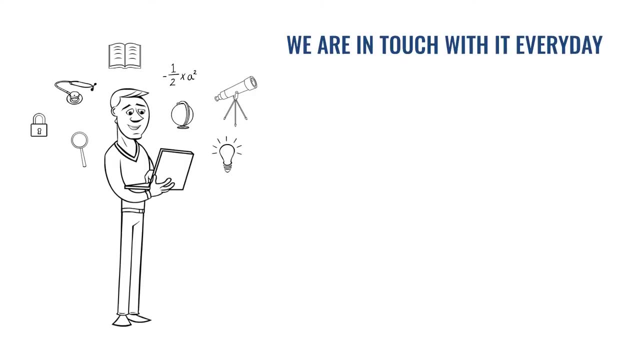 users to train the program by speaking scores of words to the system before use. Besides these simple examples, AI has been used more and more to train users to think and act like humans. In fact, we are in touch with it every day, even if we don't notice it, Whether we are. 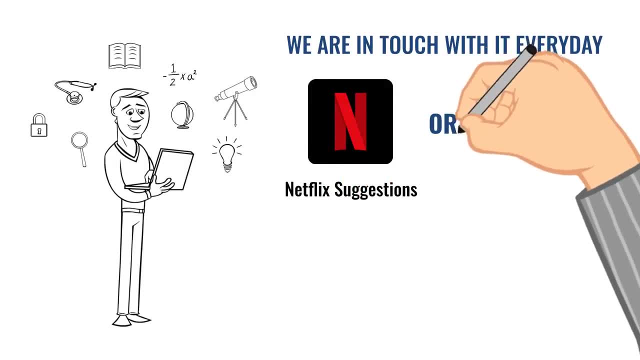 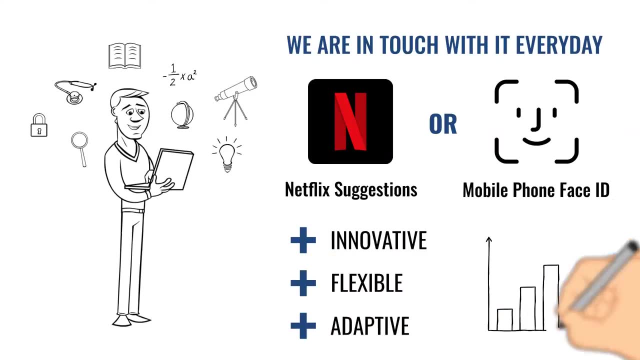 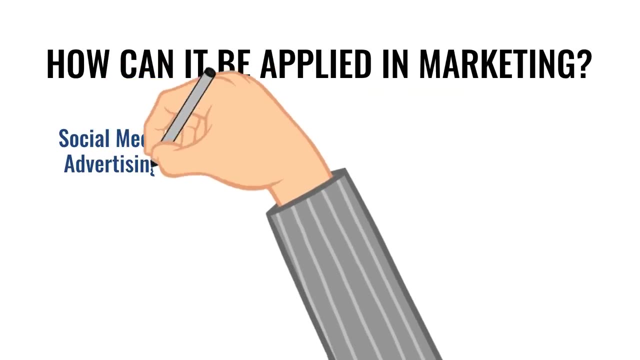 watching our Netflix movie suggestions or unlocking our phone with Face ID. AI is present and it has been allowing businesses to become more innovative, flexible and adaptive than ever. But how can it be applied in marketing? Starting with social media? Social media advertising is one of the 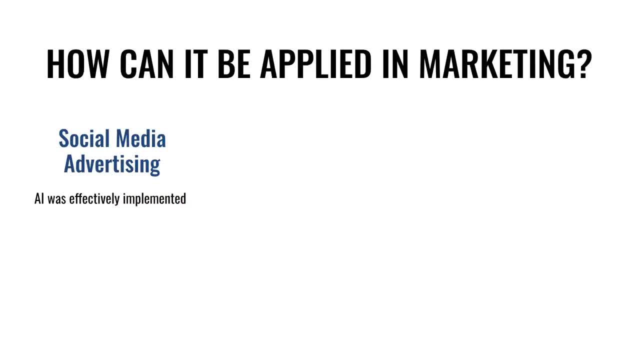 areas where artificial intelligence was effectively used. By utilizing AI and machine learning, platforms such as Facebook or Instagram can examine their users' information and interests, which allow them to personalize the content and ads that show on users' feeds. This technique is also being used by streaming platforms such as Netflix and.